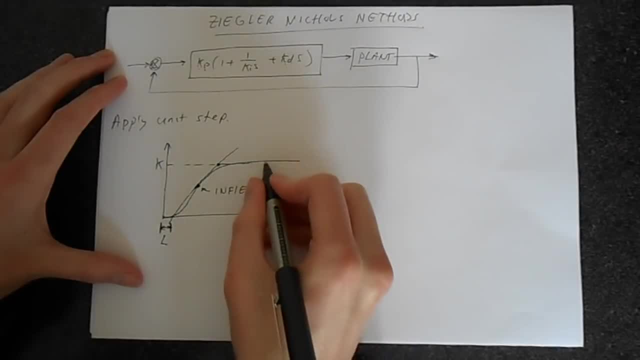 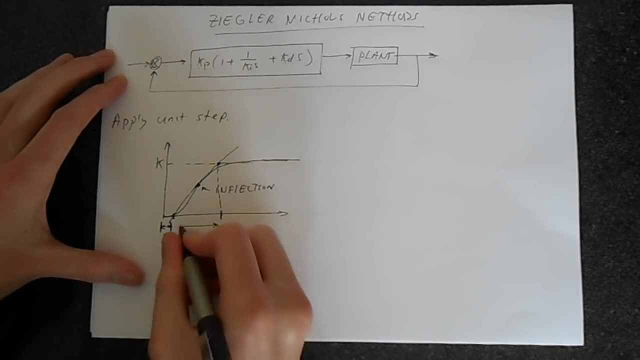 And then, if we come from where this line here, which comes along from this steady state, intersects with the tangent line, drop a vertical line down there And from this point to this point we can call this distance T And we can make up a table from this of what values we should have. 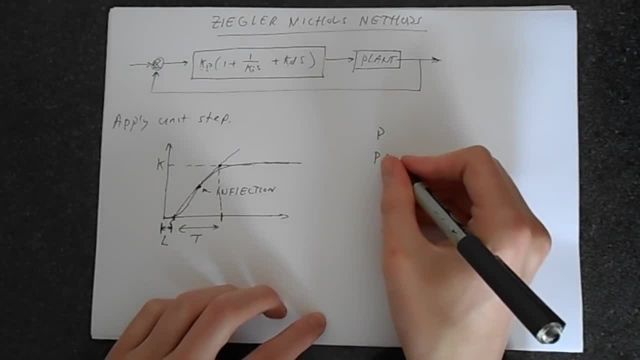 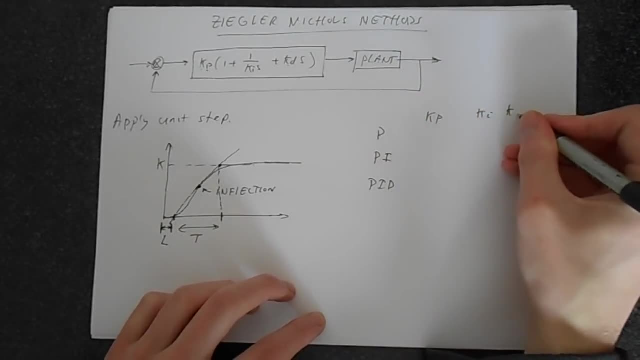 So we've got a proportional controller- proportional and inflection, So we've got an integral controller and then a PID controller, And then you've got values: KP, KI and KD. So this should be T divided by L. 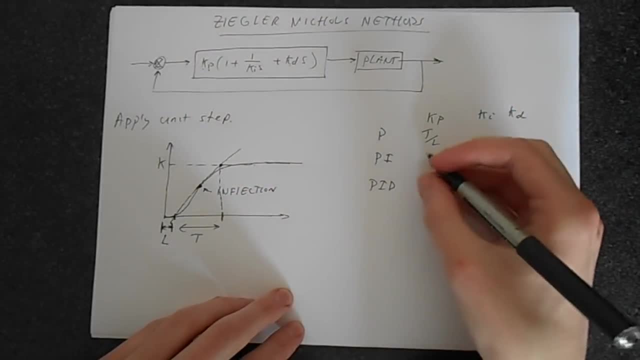 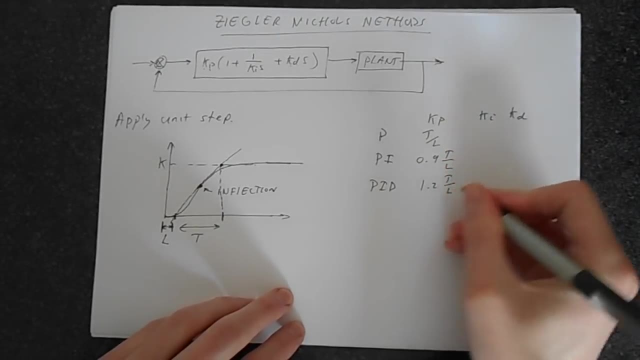 You can determine these By now. you've got enough mathematics to easily determine these. 0.9 T over L, 1.2 T over L. This one is infinity. of course That's zero. This is of course zero. 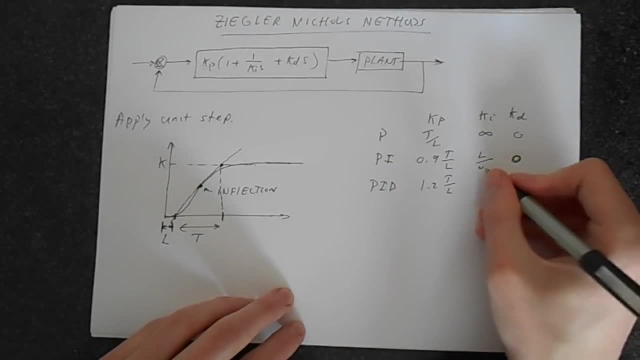 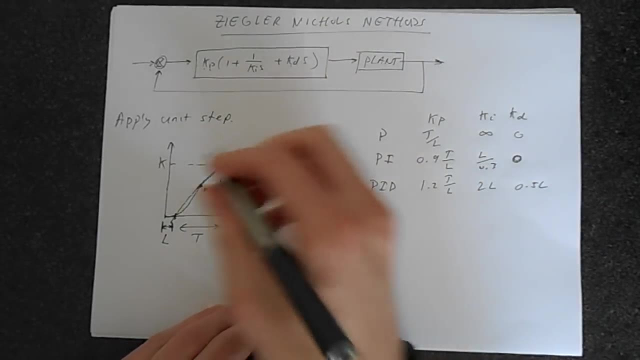 because you've got no D here. This should be L over 0.3.. This should be 2L And this should be 0.5L. So use this table once you've got your T and your L, and you get all of the values that you need. 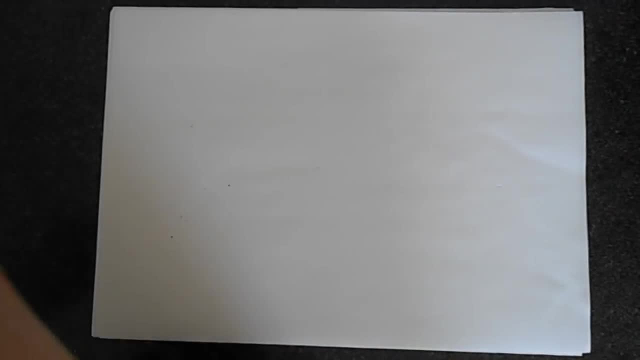 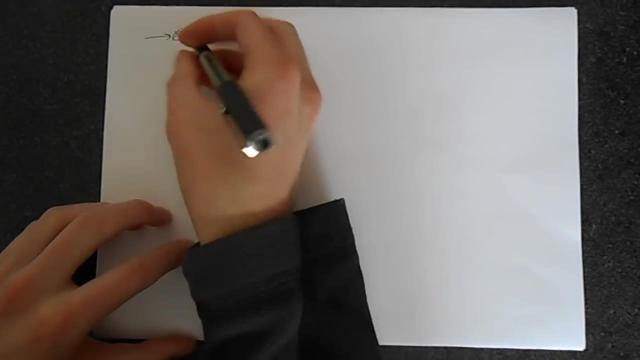 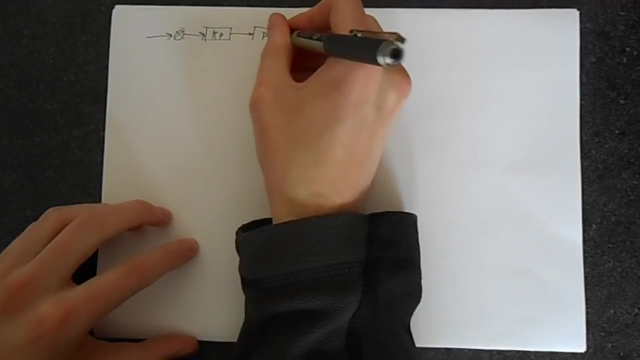 Okay, let's move on to the second method. The second method is very, very easy. It's very nice Basically set up this system. So we've got this block there, KP. Then we've got a plant Plant here. 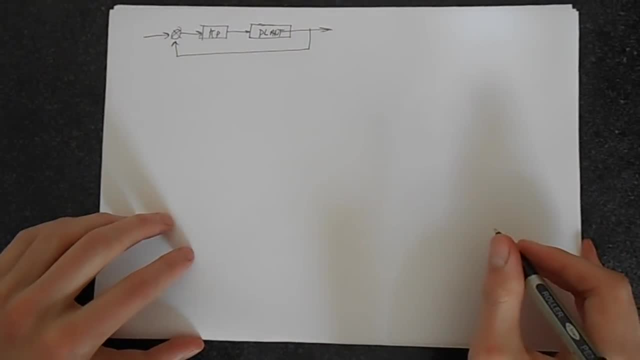 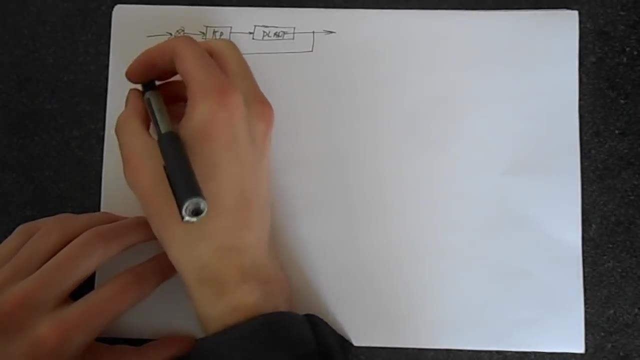 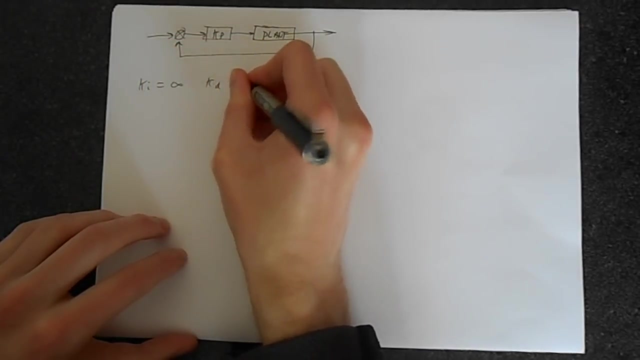 And then some feedback just shooting around. All right Now, how do we determine the values that we need for our PID controller? So let's put KI and set that to infinity, And let's set KD equal to zero. So that's kind of the system here. 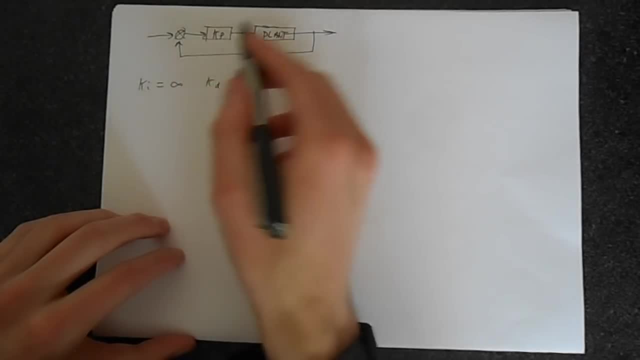 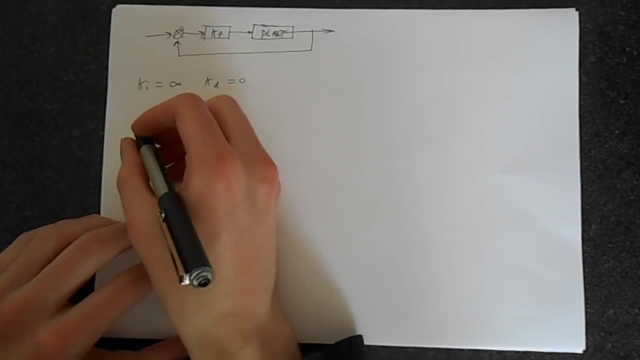 If you look at the previous system we had, you'd end up with that when you applied this. Okay, So we want to determine this thing that we're going to call Kcrit or Kcritical. This is the point at which the system becomes marginally stable. 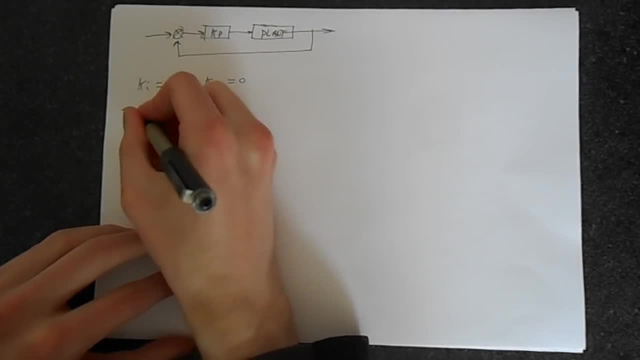 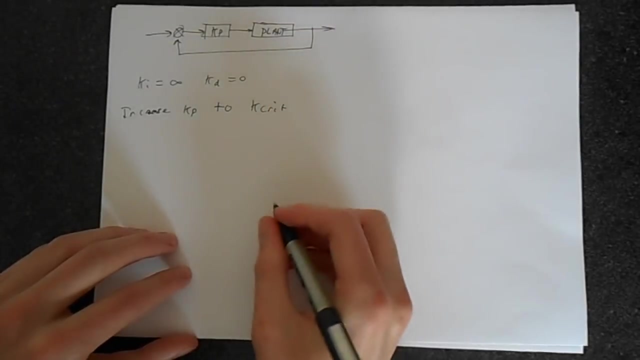 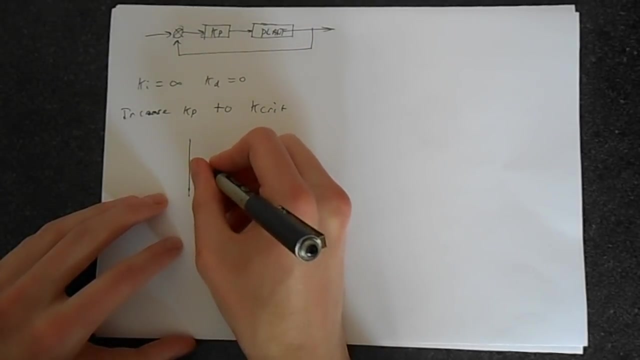 So you get a little bit of oscillation. So you increase in KP to God. I can't even spell Okay, increase KP to Kcrit, And you'll get a response that looks something like this at K equals Kcrit, Something like this: 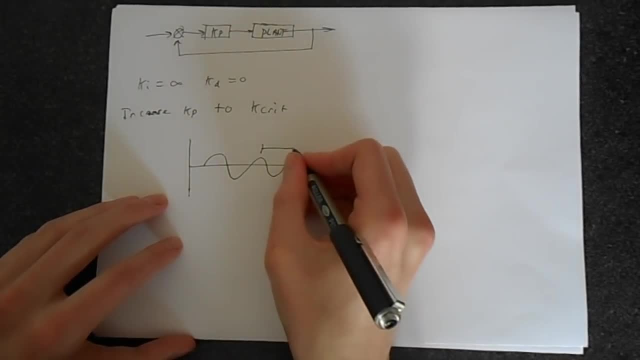 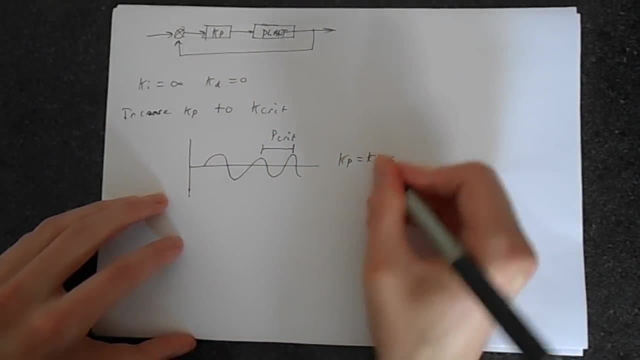 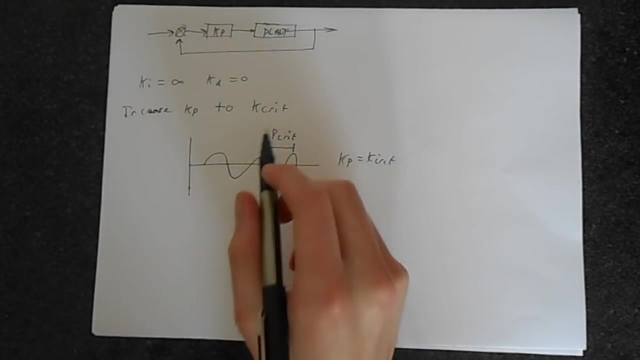 It's just started to be unstable. And you get this thing here: Pcrit, And this is KP equals Kcrit, So this is critical. Okay, Very simple, Just simulate this system increasing KP until it becomes marginally stable, So it's just first exhibiting sustained oscillations. 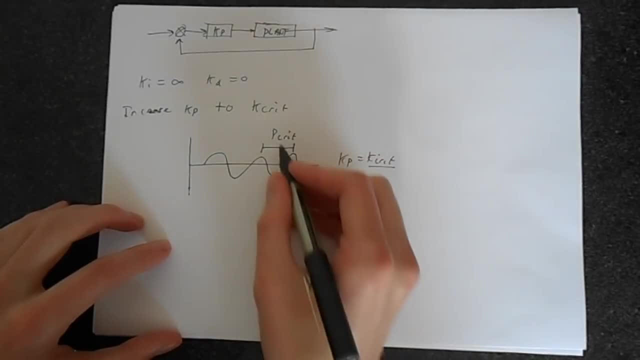 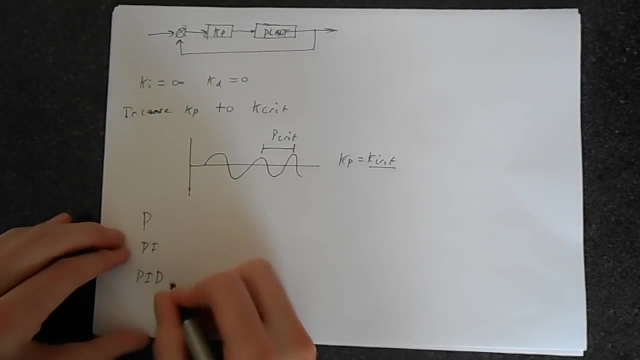 Something like this: And we have the value Kcrit And we have this value Pcrit, And then we can just get this table: P, PI and then PID. So KP is 0.5 times Kcrit. In this case we've got KD here. 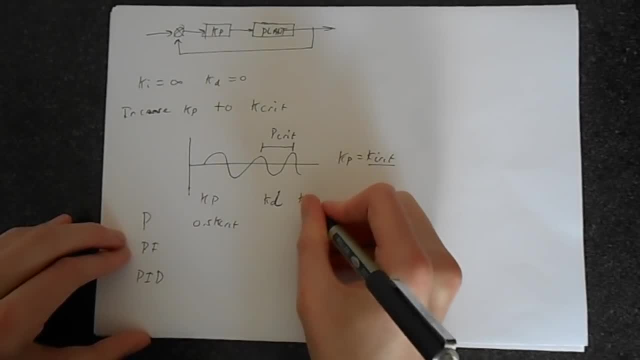 Sorry, KI, Just the way I've written my table, what I'm copying from So: infinity And then 0. Of course no D 0 here, no D 1 over 1.2 Pcrit. 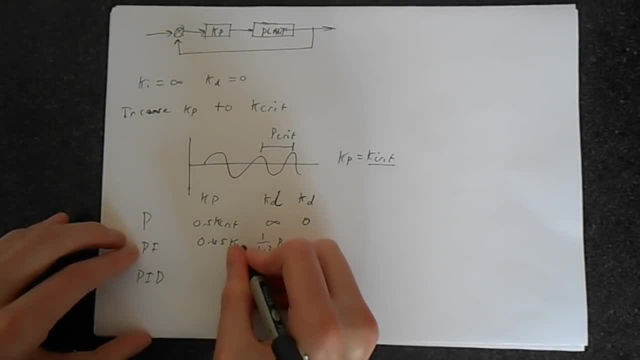 Here you've got 0.45 Kcrit, 0.6 Pcrit, 0.5 Pcrit And then 0.1 Pcrit And then 0.125 Pcrit. Okay, So that's your two methods. 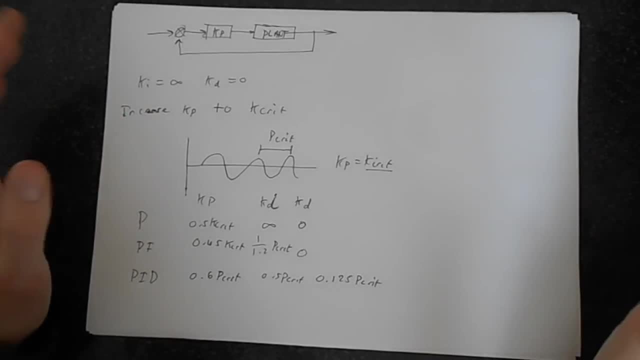 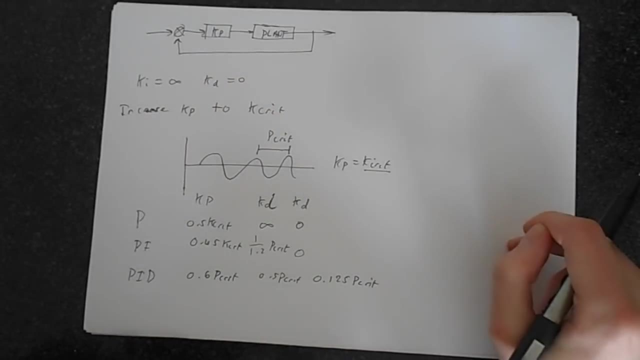 Very quick overview. Both of them are extremely simple, Very convenient to use. It has its limitations. It's not a perfect method and can only be used in certain circumstances for certain transfer functions. Hopefully this is useful to you and you can now do it. 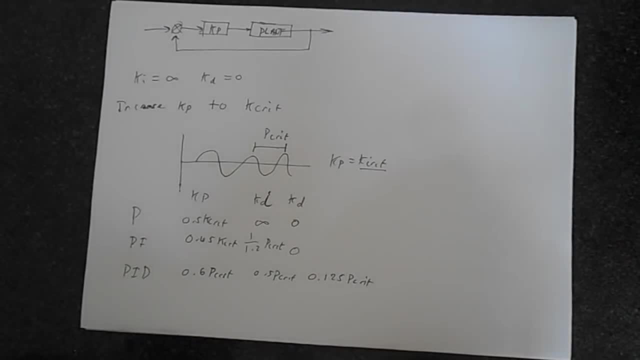 It is really simple to do And thank you very much for watching.